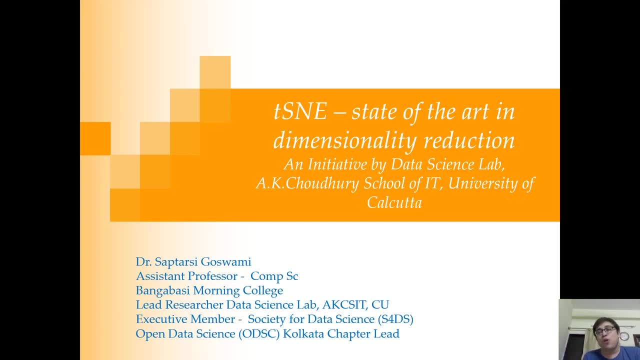 Hey guys, this is Saptarshi here and I welcome you on a video tutorial on TISNI. So it is a state-of-the-art dimensionality reduction technique. TISNI stands for T-Distributed Stochastic Neighborhood Embedding. I am sure the 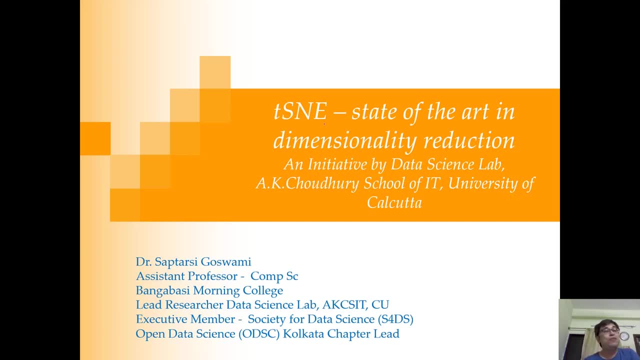 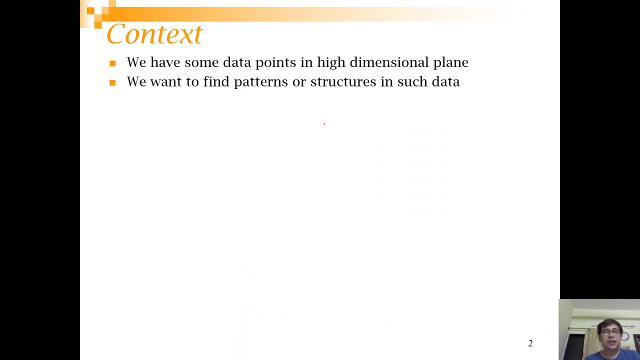 first reaction is not going to be very pleasant for you when you hear the full name. But please bear with us. we will try to make it as simple as possible. So let's set some context. Let's say that we have some data points in high. 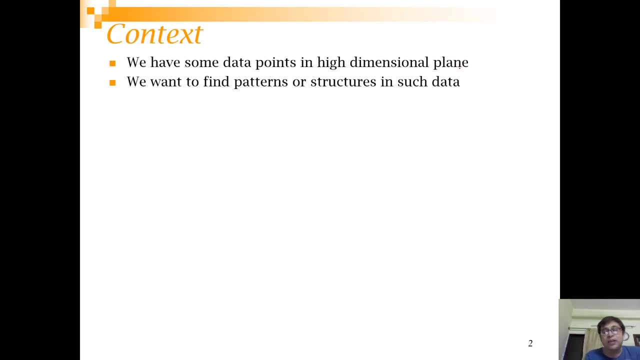 dimensional plane. So you know already that. you know, in case of text or image by informatics, recommendation system, individual observations, has more than 10,000 features, 1000 features, 1 lakh features, Okay, and you want to find some patterns or structures in the data. So it is not at all trivial, Okay, so one of the 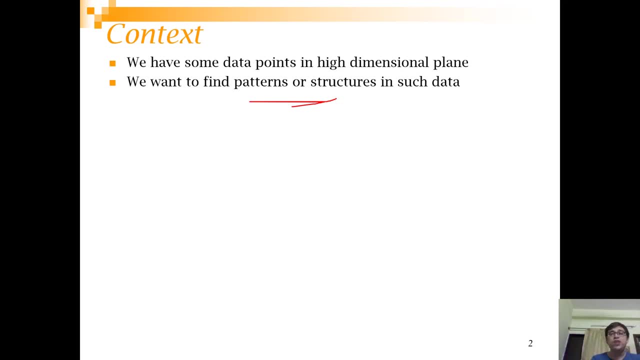 things that can be done is that reduce these 10,000 features to two or three features and then draw them in a scattered block. Okay, and we can definitely find some pattern in that. So PCA and LDA tries to reduce dimensions and how it tries to do is PCA tries to find. 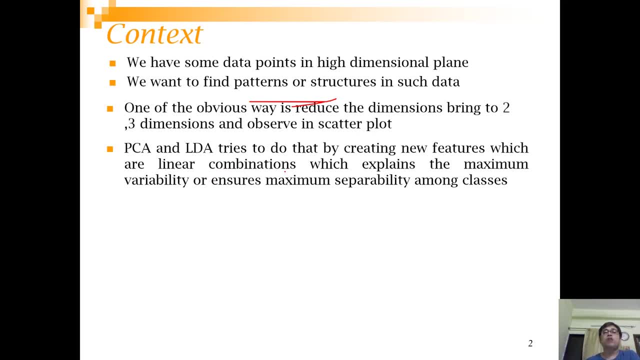 new features such that there linear combination of original features which explains maximum variability in the data. LDA tries to ensure minimal maximum separability among classes. So it is a supervised technique and needs the class levels. This need takes a different view. So let us try to understand that with a diagram. So let us say: 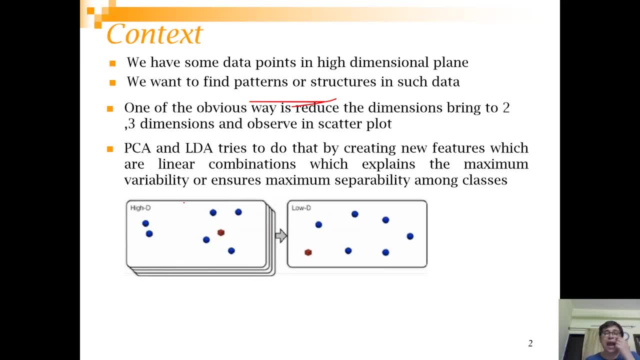 you know, these are the points in high dimension. So as in high dimension it is very difficult to visualize. So we have plotted in two dimension. only. Assume that it is in high dimension and we want to plot it into lower dimension, such that the locality or the neighborhood structure. 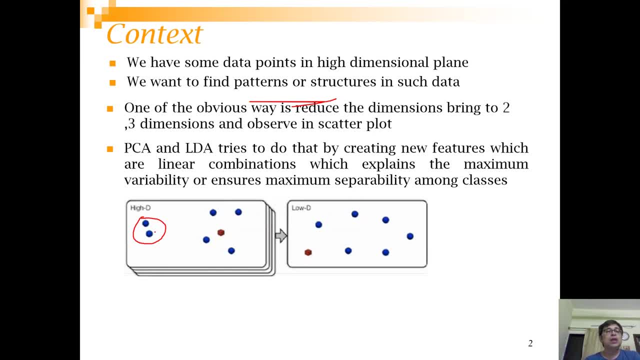 is preserved. So what do we mean by this? We mean that if this point is the nearest point or nearest neighbor in high dimension, this should be preserved when we take this to low dimension or a two dimension plane. And this is not only true for this point. this should be true for 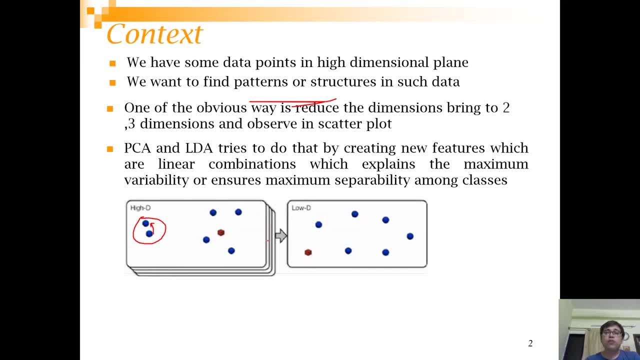 all other points, All right. So if you look at this particular representation, you can understand that this doesn't qualify or this doesn't have such a characteristics. However, if you look at a data like this, you know this actually preserves the neighborhood structure or the neighborhood. 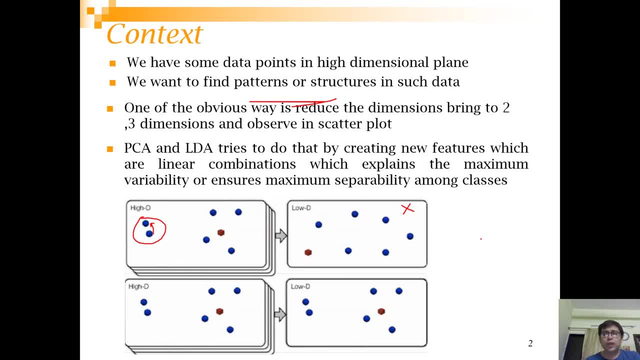 information. So this technique, one of the brains behind this technique, was Geoffrey Hinton, who is a professor at the University of New York. He is a professor at the University of New York and he is also the founding father of deep learning and many other theories. So this paper, the original paper, the first paper, was named as S and E Stochastic Neighborhood. 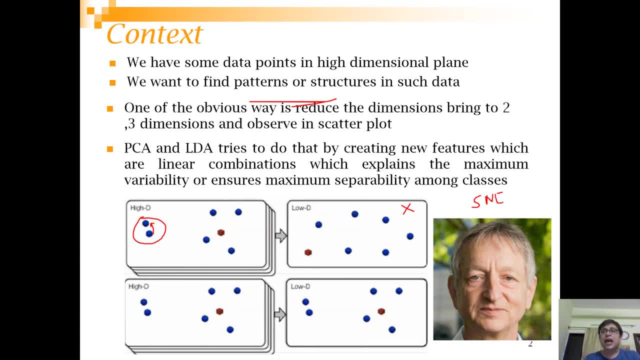 Embedding. So this is what we are going to study first, and then it was extended to something called as TISNI. This was published in JMLR, Journal of Machine Learning Research, as I mentioned earlier, also one of the top journals of machine 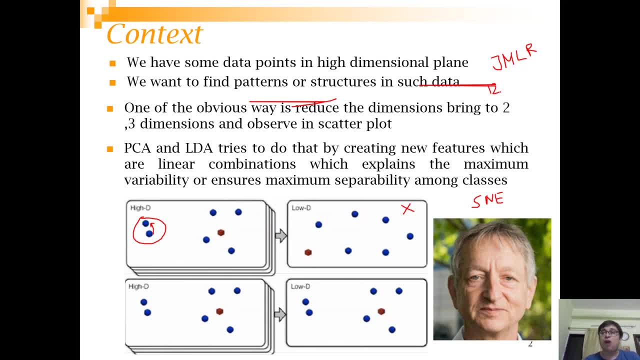 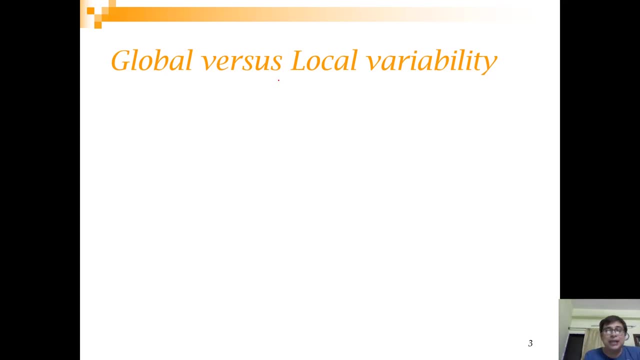 learning. This particular paper itself has got more than 12.5k citations, So highly recommended to read. So now let's understand this. global versus local variability. So, as I said, that PISNI tries to preserve the local neighborhood structure, So what PCA tried to do? PCA tried to maintain the overall variability of the data. 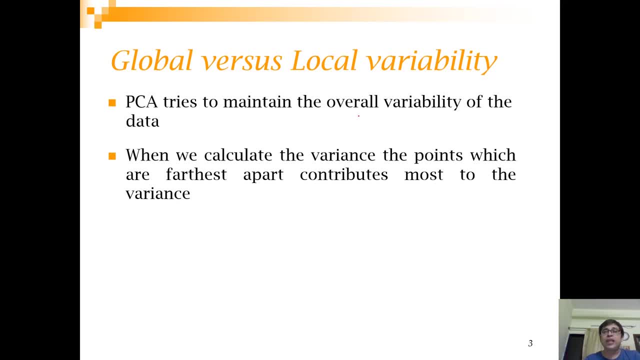 And I am sure you will agree that the overall variability can be best represented, or most easily represented, by the variance of the data. And if I think of the variance, variance is nothing. but you know, the squared distance from the mean- You know the furthest points- actually contributes most to the variance. 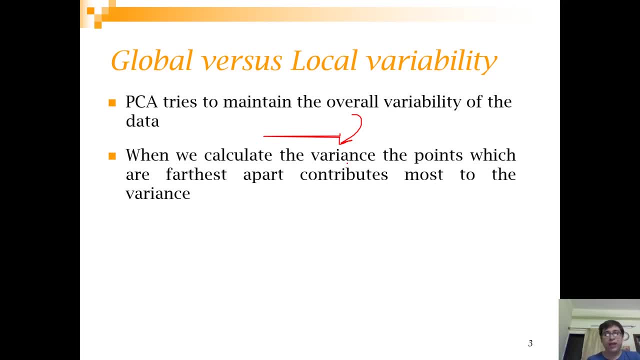 So they have the highest distance with the mean. So that's it. We can say that PCA tries to maintain the large pairwise distances. So this is why you know, we will say that PCA has a global focus. So it is looking at distances, or trying to preserve those distances which are far from 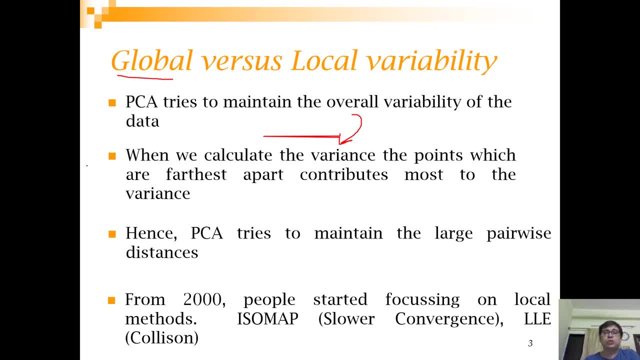 each other. From 2000, actually, people started focusing on local methods. They thought that this- you know, large pairwise distances, which are global Distances, may not be the best way to represent that particular data set and that may not be very stable as well. 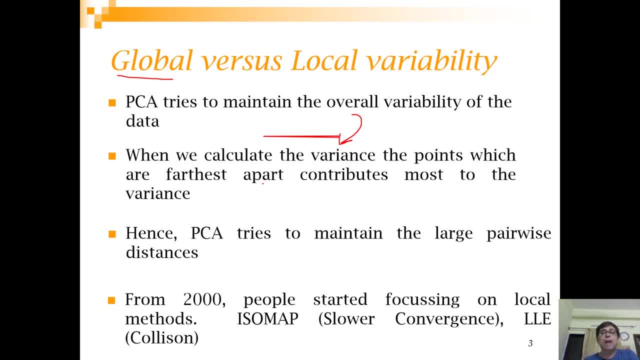 So they started focusing on local methods. Couple of local methods are ISOMAP and LLE. So LLE stands for Linear Local Embedding, So both came around the year 2000.. So ISOMAP had a problem of slower convergence. 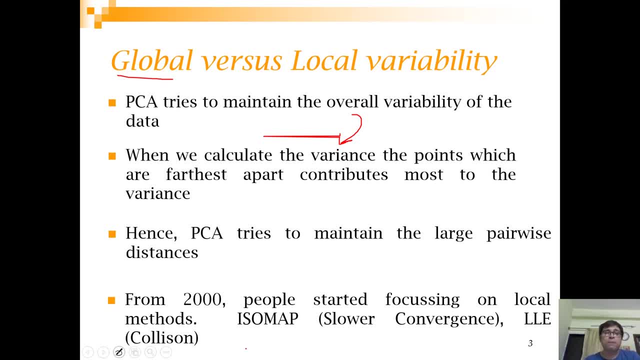 Whereas LLE had a problem of slow convergence. So they started focusing on the local methods. They thought that PCA had a problem of collision. So what do you mean by collision? So as we move from higher dimension to lower dimension, it may so happen that you know several. 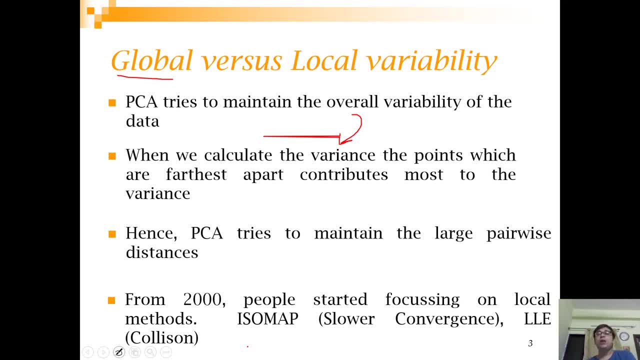 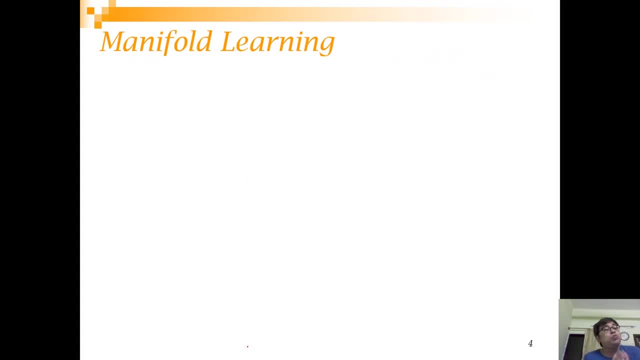 points of higher dimension gets converted to the same point in lower dimension, So that would be called as collision. So now, this was one of the issues of PCA, that it focused on global learning. Another problem was that it didn't understand many folders. So what is many-fold learning? 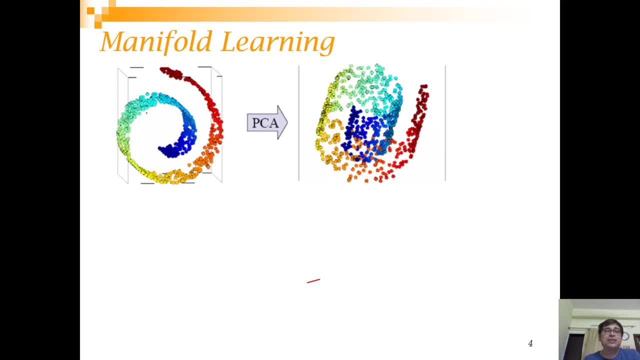 So many-fold learning is best illustrated by this Swiss rule. So you can understand that the points which are in the same curvature, they are similar. So that has been color coded similarly appropriately. So if you apply PCA and then you know, in this reduced dimension you plot them by the original. 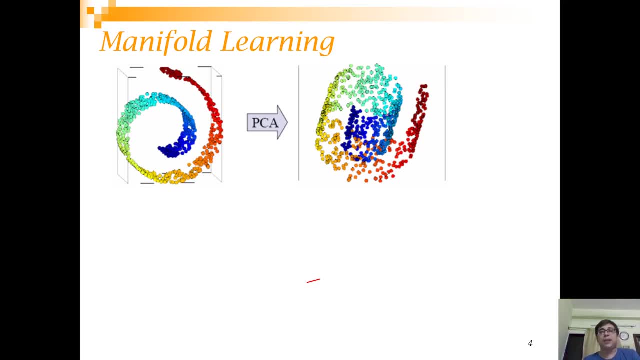 colors, So you can see that it has gone all over the places. So this separability is no longer maintained. So there is a concept, and this happens because PCA focuses on Euclidean distance. So what is Euclidean distance? So Euclidean distance is actually, you know, if you look at these two points, 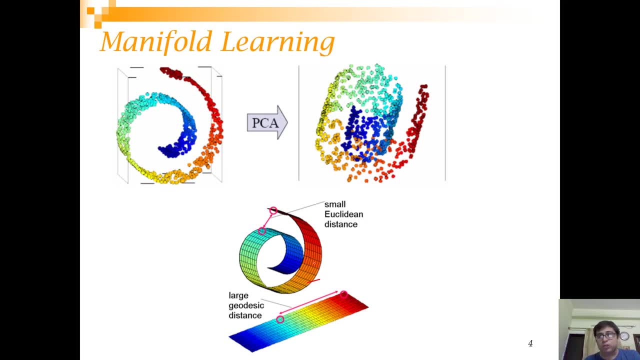 So they have small Euclidean distance. similarly, you know, here also there can be small Euclidean distance, But they are from completely different curvatures. So instead of Euclidean distance, if you consider geodesic distances, So these will be appropriately, you know, stretched out so that you know points from different. 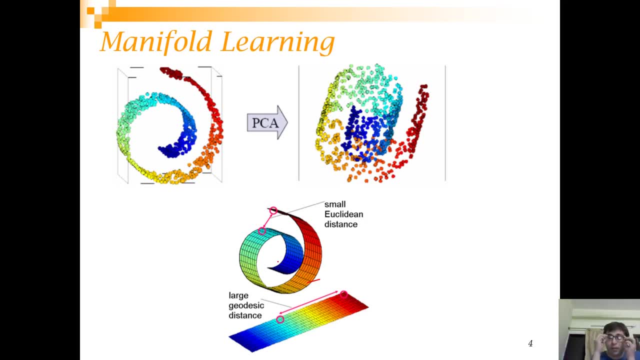 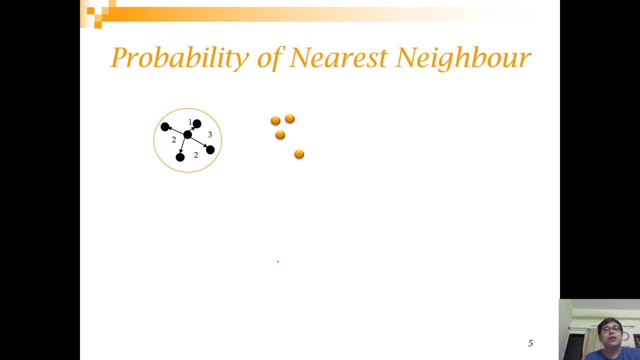 curvatures, different curvature equations will be further from each other. So, with this knowledge, now let's look at, or let's try to understand that, how we can try to represent this neighborhood information. So let's take a simple example. Let's assume that this is in higher dimension. 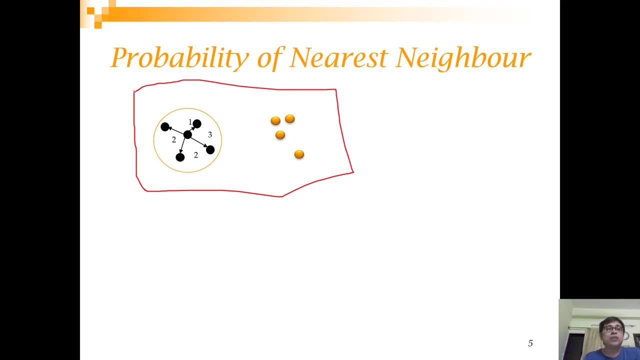 And these are, let's say, nine points that are there. So this is your reference point. This is your reference point, And what I want to do is I want to represent this point in terms of its neighbors. So how can I do that? 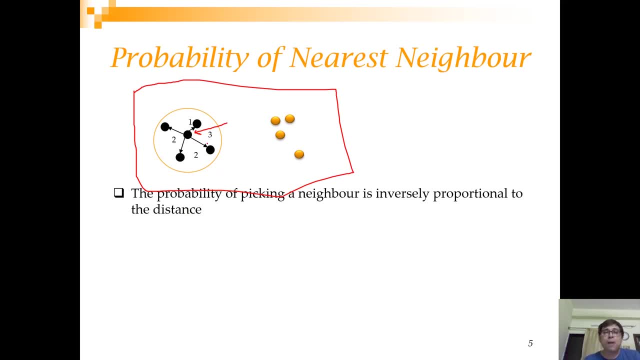 So what I can do is I can first look at the probability of point. What is the probability of picking this neighbor? okay, So let's say this neighbor has been picked for lower dimension. So if this neighbor has been picked, what is the probability of this neighbor being picked? 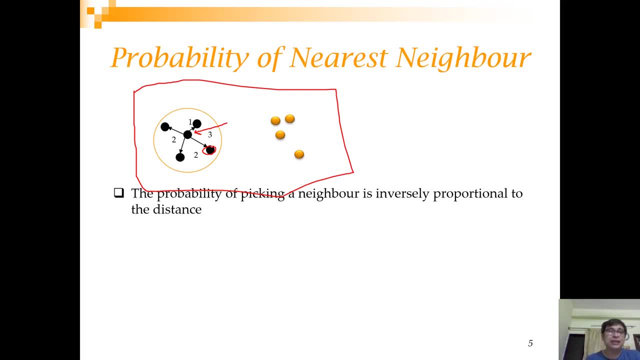 okay, And you will agree that this should be an inverse function of the distance. One such function is this exponential function and if you use this exponential function, okay, this is similar, These are similar characteristics. So this is the exponential function. This is similar characteristics with a Gaussian distribution. 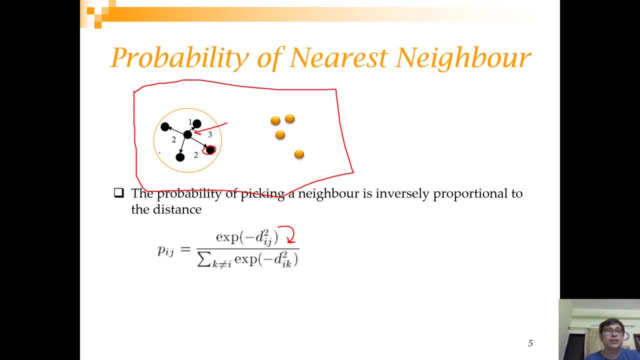 So you can think of that. this point, you know, around this point there is a Gaussian distribution, okay, And what happens is that as you go farther away, so for these points, okay, the probability of picking this up will be very close to zero. all right, So you know, this can be seen as that. you know these were the distances, if this is a reference. 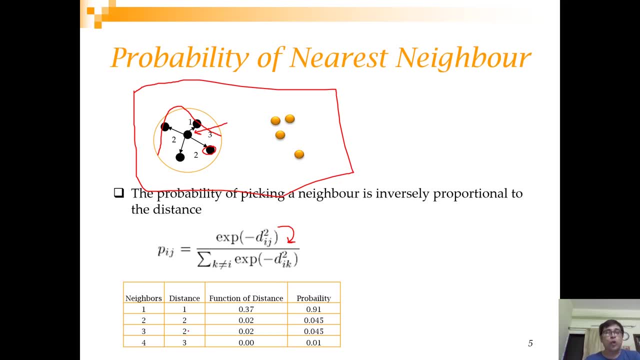 point. the distances are 1, 2, 2 and 3 respectively. So if you apply this, If you write this function on the distance, okay, so you get a value like this, all right. And if you convert, so if you find the probability using this formula, okay, you get a probability. 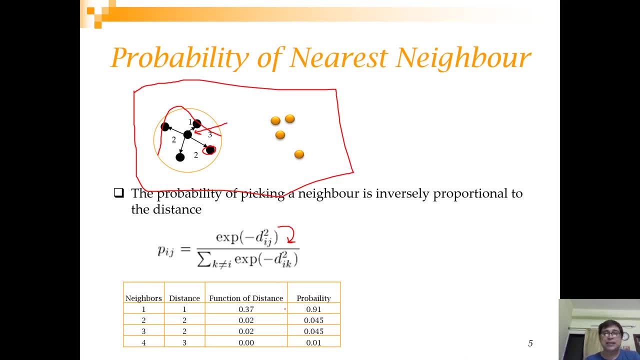 like this. So you see that the one that was the closest has the highest probability, and then you know the probabilities has reduced further. all right, So you see that earlier you know this was a vector in hundred dimension. So if you convert In hundred dimension now, this can be thought as a probability distribution. 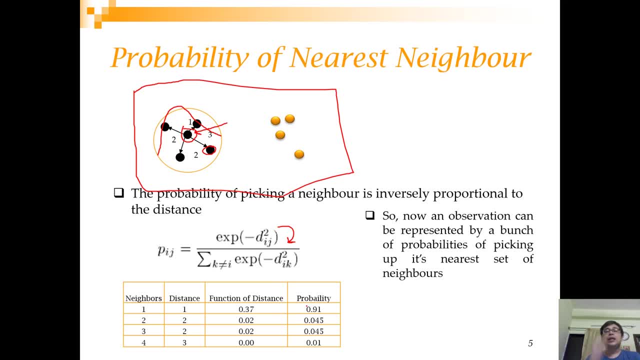 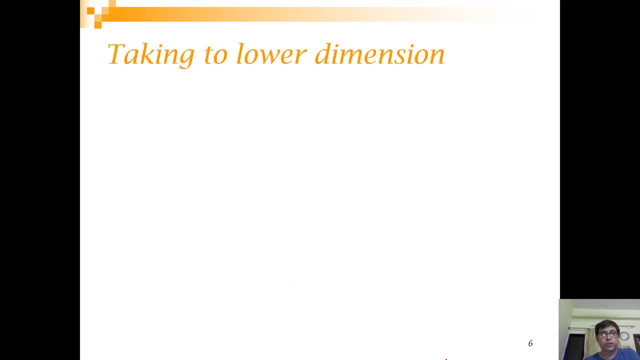 What this probability distribution actually represents. The probability distribution represents the probability of picking its neighbors. given that this has been already chosen, okay, So, as I said, the data matrix can be converted to a probability distribution. all right, So now let us say that we have some means, okay? 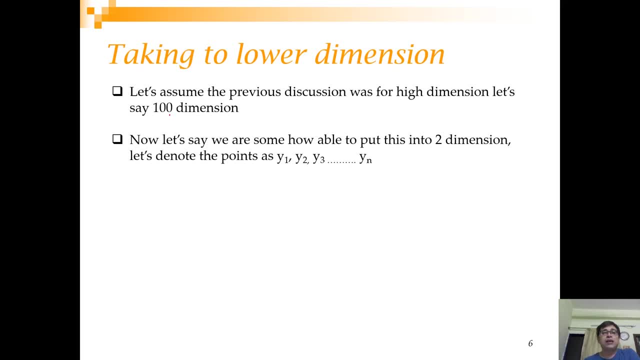 Some magic trick. by which? magic trick by which, in the from the original hundred dimension or thousand dimension plane, we are able to go to a two dimension plane? okay, and in this two dimension plane we represent the points as y1, y2, yn, like this, all right, and you know, we let us assume that we had. we had k. 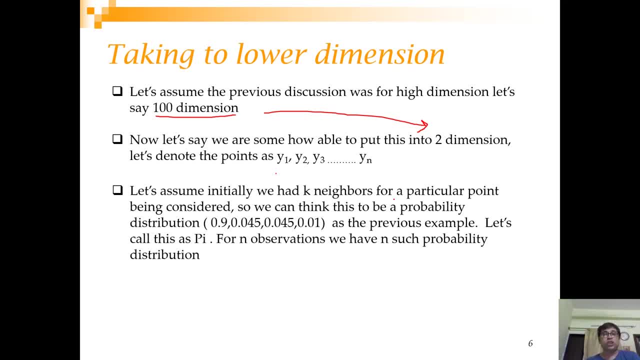 neighbors. okay, based on based on the Gaussian function, so we can think this to be a probability distribution. so, the example that we discussed, instead of that hundred, a vector with hundred features, I can represent it as a probability distribution and let us call this as p, all right. 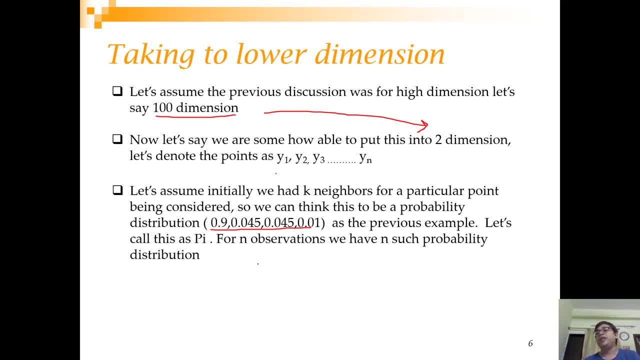 so for n observations, we have n such probability distribution. okay, and in same manner, let us compute this probability distribution of each of the points in y. okay, so we are doing the same thing, what we did in the original dimension. we are picking the same point in the original dimension. 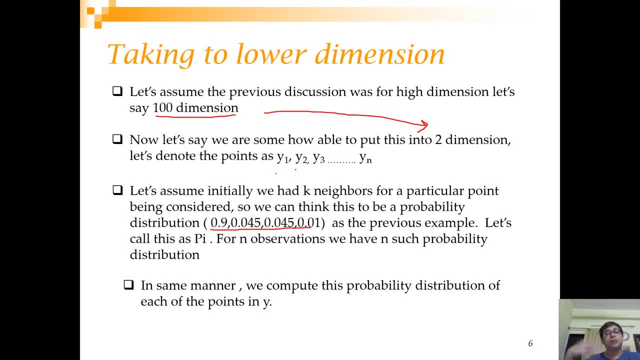 or, or, or the representation, lower dimension, representation of the same point, and then we are trying to pick up the neighbor and calculating the probability. okay, and we are, you know, using the same Gaussian formula. okay, now we have another probability distribution, so we have one probability distribution corresponding to the original feature space which you are calling as p, and this we are. 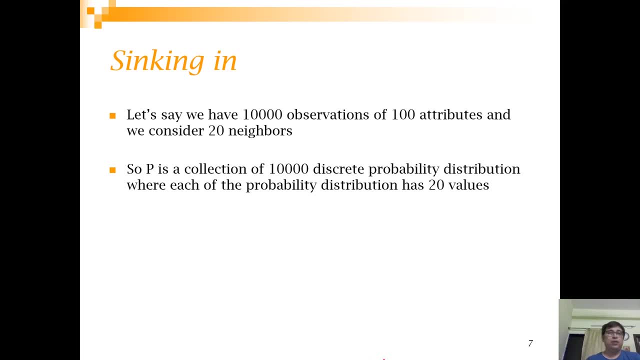 calling as q. let us think this further. okay, so let us say that have 10,000 observations of 100 attributes and we are considering 20 neighbors. okay, and so now p is a collection of 10,000 district probability distribution. so for each point you have a. 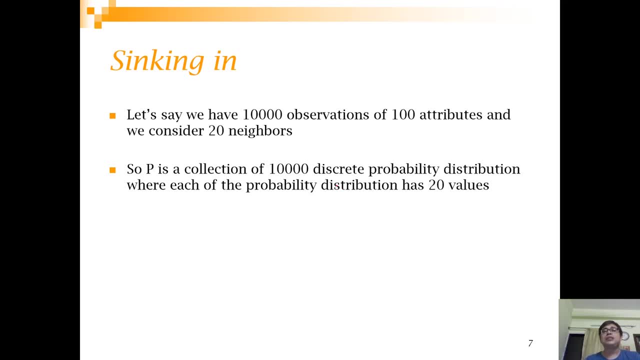 district distribution and each of them has 20 values, because- because you are considering 20 neighbors and, as we said, that let's buy some magic or tree- we have converted into two dimension distribution. now also we have a probability distribution. these two probability distribution- dimension wise at least- are of same nature, right? so both have, both are collection of 10,000. 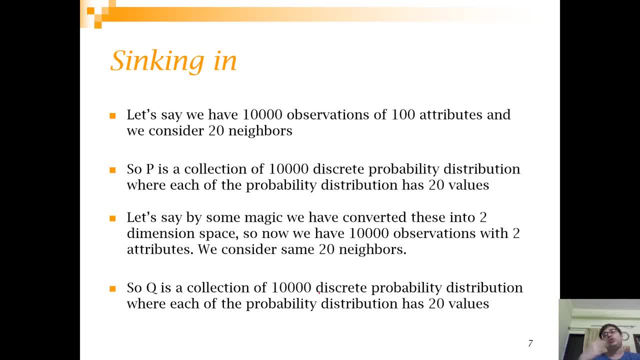 probability distribution and individual distributions has 20 values each. so can you tell me that what should be the relationship between p and q? okay, so we can think about similarity between p and q. so we have seen that how we can can measure similarity between two vectors, but we have not seen that how we can measure. 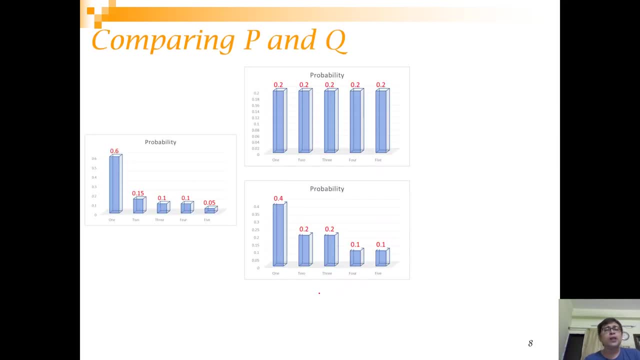 similarity between two probability distribution. so let's have some intuitions. so let's say that i have in my original feature space. i am looking at one point. let's say i and i am, my k is 5 and i have a probability distribution like this, when i have taken this to a lower dimension: 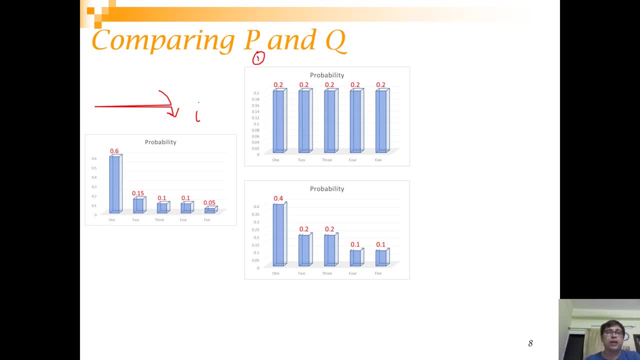 okay, so this is one possible representation in one lower dimension and this is one possible representation in one lower dimension. okay, so this is one possible representation in one lower dimension, dimension, and in another toward dimension. this is another representation. okay, so you know what we want. okay, uh, so let's try to- uh, you know uh, first represent this in. 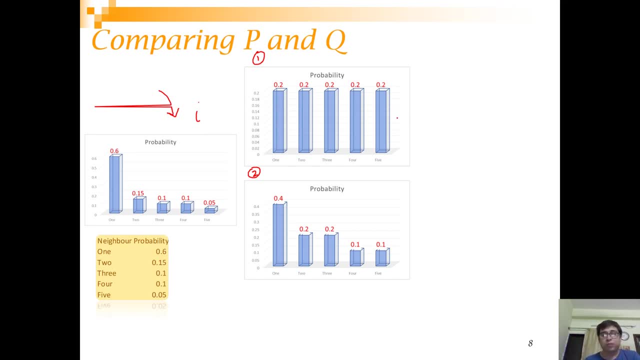 terms of a table, and also this in terms of a table. so first, what we do is let's find a ratio between, uh, you know, uh, the first neighbor of both these probability distribution, okay. so 0.6 by 0.2 get a 3, 0.15 by 0.2, i get 0.75. that okay. and similarly, let's do the same for this quality. 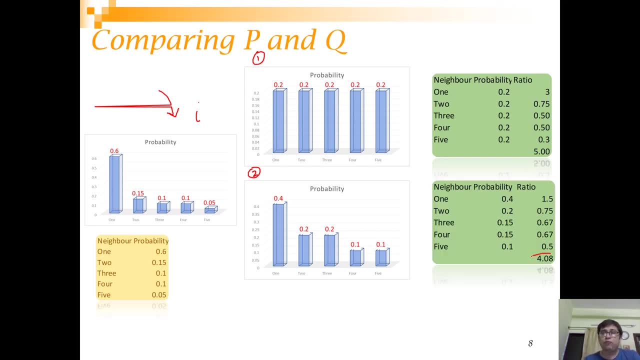 and if i do the same calculation, you will see that the value here is 4.0. and if you run several example, you will see that if the probability structures are similar, then you know, uh, this sum of these ratios will be lower. so if i use a function of this sum of ratios, okay, uh, so that can work as a similarity. 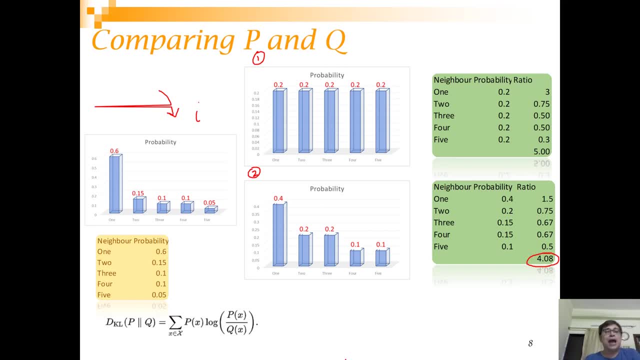 measure between probabilities. so this is formalized in a very popular measure called as kl divergence. okay, so, which is a function of this px by qx which we discussed. then we are taking a log and also multiplying by the probability in the original feature space. so this is about one point. 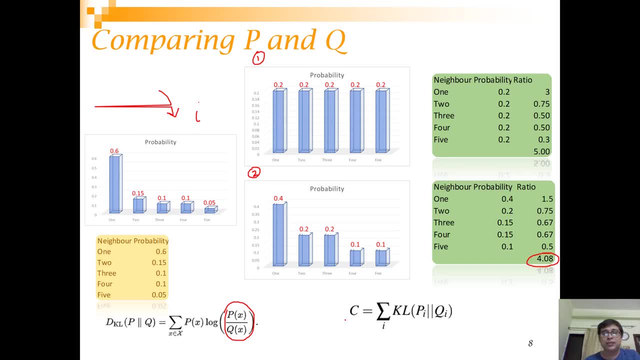 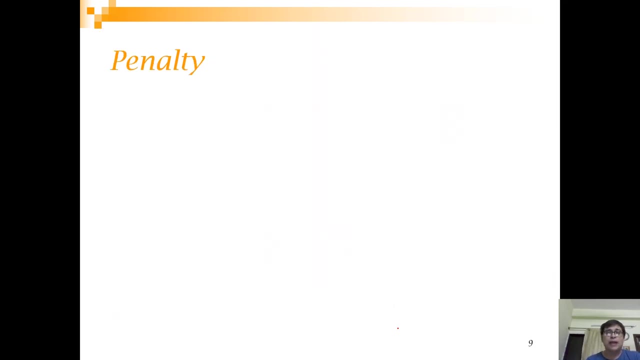 so when we calculate about all that 10 000 points, we represent that as c, and here your i is 10 000. okay, so of course you want to minimize the value of c, all right. so, uh, now let us look at this. uh, particular function. okay, and let's see that how. 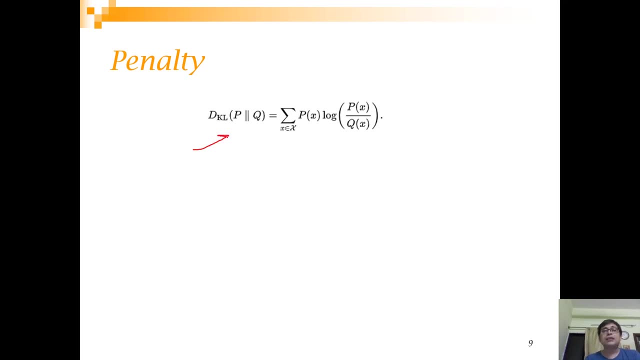 you know this is good for preserving the locality or preserving the neighborhood info. So let us take two cases. So always you want this ratio to be small, So you want either this to be similar or you want px to be small and qx to be high. 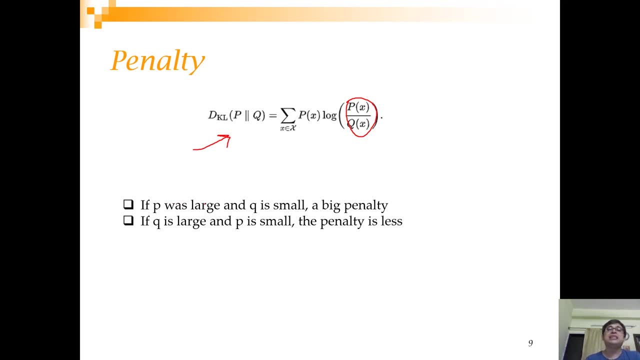 So let's take a case where p is large and q is small. So what does that mean? So p is large means that in your original feature space this was a quite close neighbor. However, q is small. That means that in lower feature space you could not preserve that information. 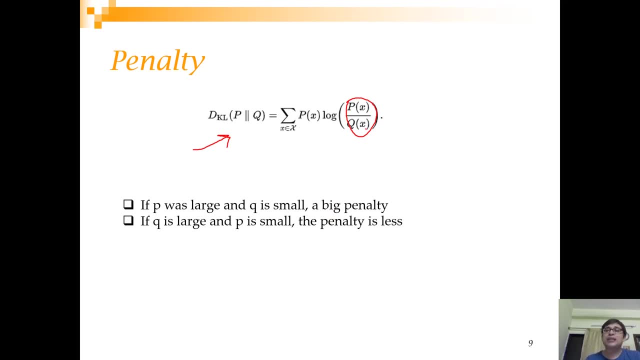 So this ratio will be high. So that means that c will be higher. So you want to minimize c, So it will result in a big penalty. So whenever it tries to find this q, it will always try to keep this ratio. However, let's take the other case, that q is large and p is small. 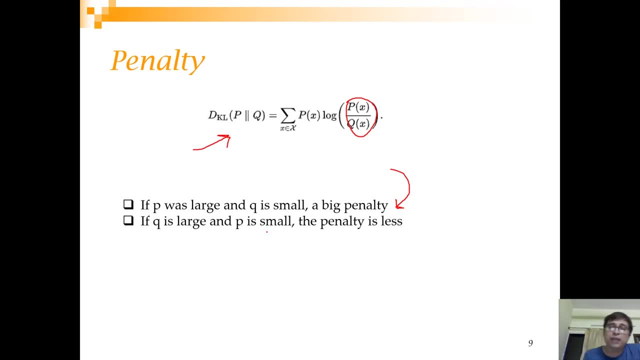 So in original dimension they were far apart, But in the lower dimension they are quite close. OK, so this simply doesn't care much about that. So that's why we say that you know it can preserve locality and it ignores global information. 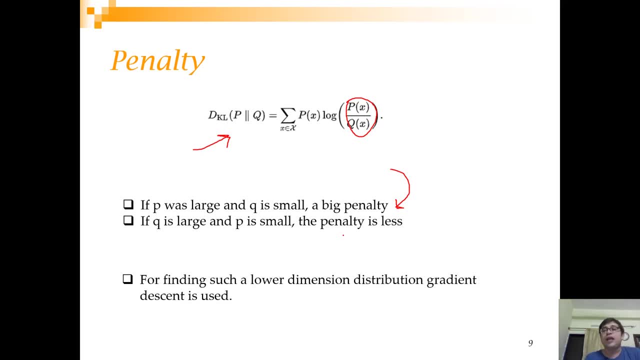 OK, And for finding such a lower dimension distribution, we have to find the lower dimension distribution. We can use gradient descent, one of our, you know, master keys, as we have discussed in one of the previous lectures. So we have discussed only the mathematical intuition. 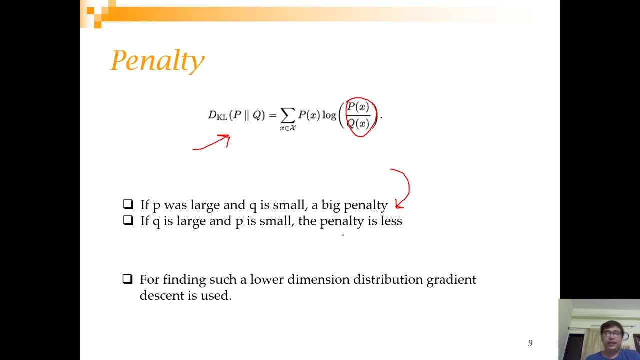 So we are not going into how you solve using gradient descent, All right. Now there is something called as a perplexity, So we talked about, if you remember that, selecting some neighbors. OK, so how to select some neighbors. So actually, you know, we talked about distances. 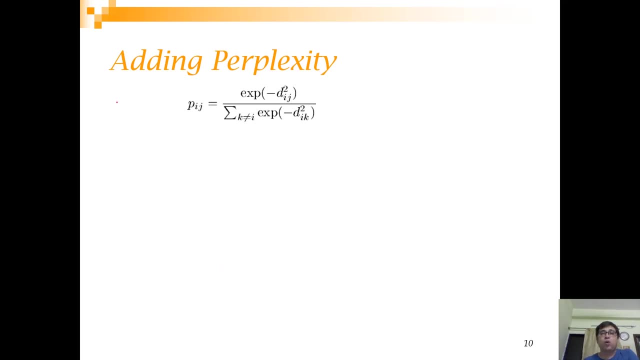 And we kind of we did not go into discussion that what this distance actually looked like. OK, So it may not be your Euclidean distance. One of the popular choices is a distance like this, which is called as kind of a scaled Euclidean distance. 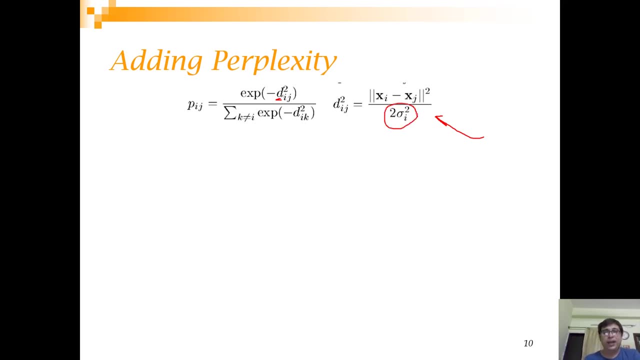 which is, you know, divided by the variance. All right, OK, So if you have a, you know, distance like this, this actually, you know, works as kind of a setting of a neighborhood. OK, So this perplexity actually determines how many neighbors will be considered. 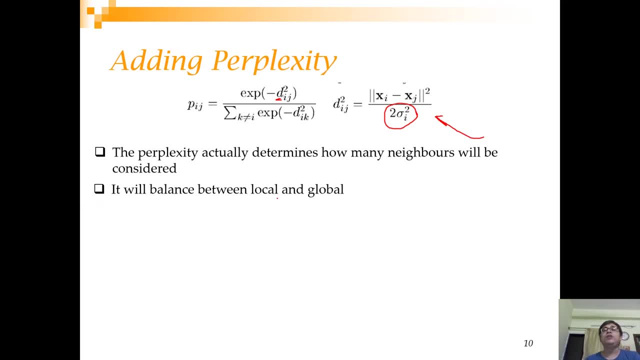 OK, And that that way it can balance between local and global Right. So if you have small number of neighbors, you know you are local, And if you have taken a lot of neighbors, then you are slowly going to the global, global structure. 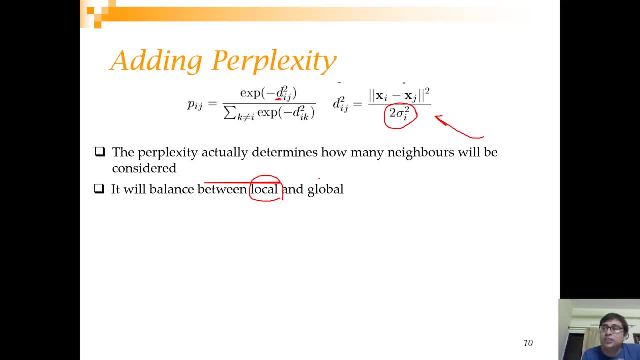 All right. So in the original paper the authors have mentioned you should have a perplexity between 5 to 50. So let's look at some examples. So let's say that you know in original dimension. So again for simplicity, we are even taking the original dimension also in 2D. 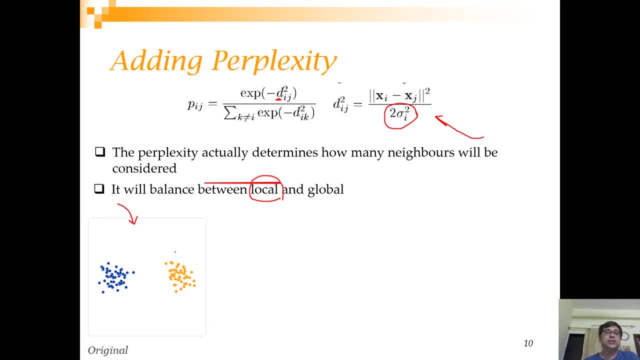 So these were two set of distributions. So you can see that. you know they come from different Gaussian distributions. OK, So if you have a low perplexity, you know this is what the representation in 2D. OK, So what do you see? 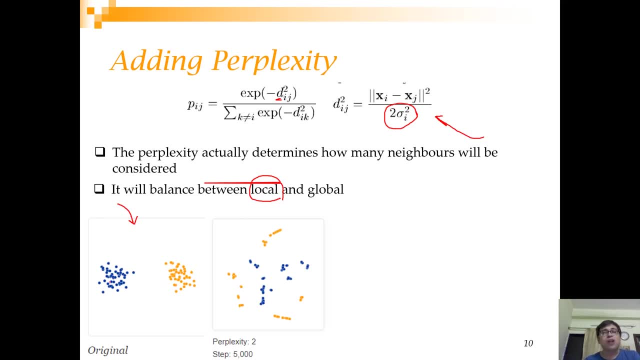 So actually it has focused a lot on the local structures, OK, So it might have, you know, looked at some structure like this or some structure like this, OK, And you know, this is how the lower dimension representation looks like. 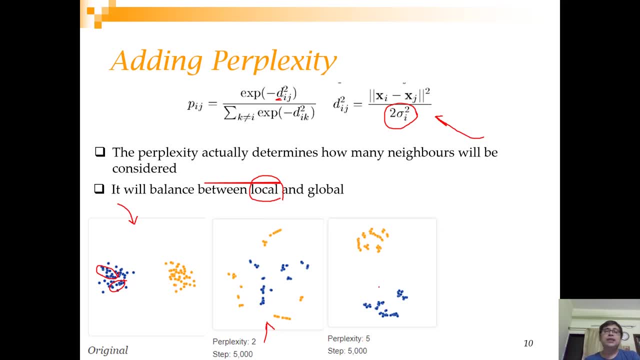 If you go to a perplexity of 5, this has now nicely identified the structure- OK. And if you increase the perplexity beyond certain point, OK. So this is just as an illustration. So here we have taken a perplexity which is even more than the number of points that are there. 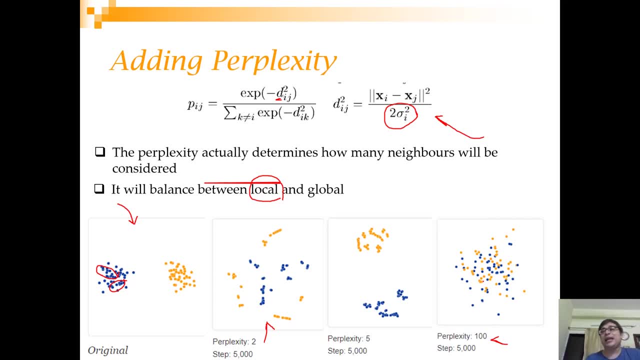 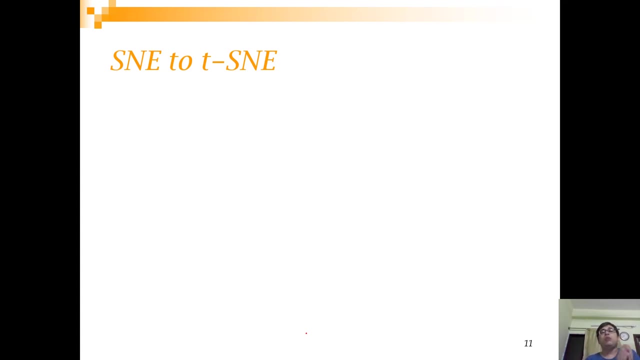 OK, In this example. So this can again become quite, quite random. OK, So the perplexity should be not very small and not very high. OK, Now let us try to understand. So this was all about stochastic neighborhood embedding. 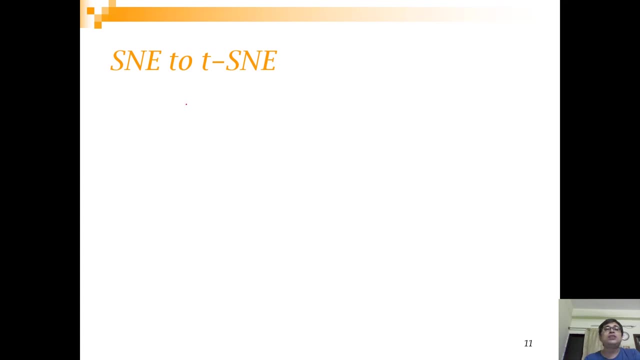 OK, Now let us try to understand that. What was the motivation between T and SME? OK, So you know, this was the probability distribution that we were using in the lower dimension, Right. So, as I said that this follows kind of a Gaussian distribution. 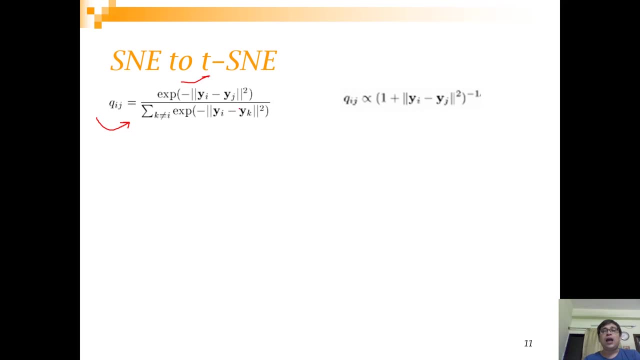 This was in SME. In T and SME a different formula is used. The formula is something like this: OK, And actually, as this representation, this represents normal distribution. This actually represents students T distribution with a degree of freedom one: OK, So that's why you know, as T, SME in the lower dimension follows this probability distribution. 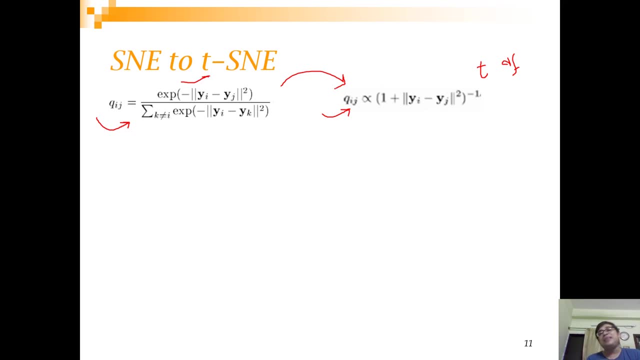 OK, You call this as T SME. Now an obvious question that should come to your mind is that: why do you follow T distribution? So let's try to tell that. So of course you know you want to preserve local distance. 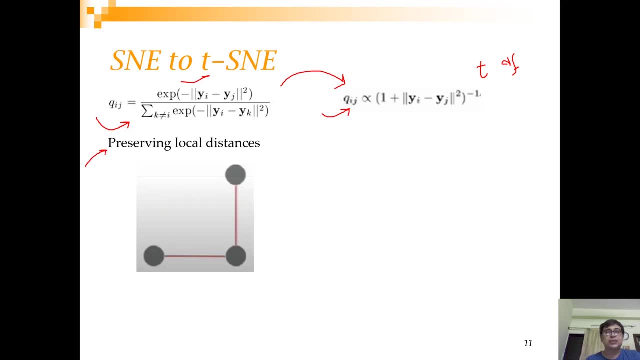 OK. And while you are preserving local distance, OK, So you also want to do something else. So let's look at this example, Right? So what are the local distances? So you see that you know this can be considered as local distance. 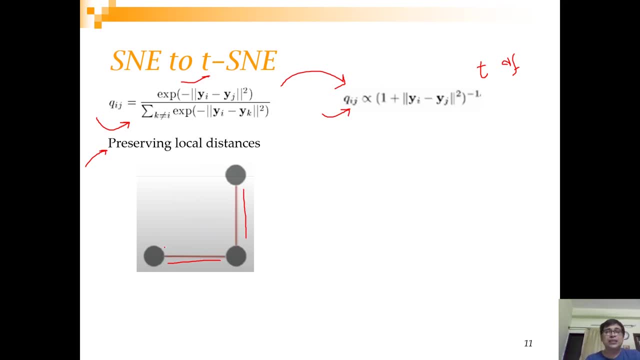 OK, So this is in 2D plane And this is the farthest distance, So this I call as a global distance. OK, To simplify, Right? So these two pairwise distances represent: This represents local distance and this represents global distance. 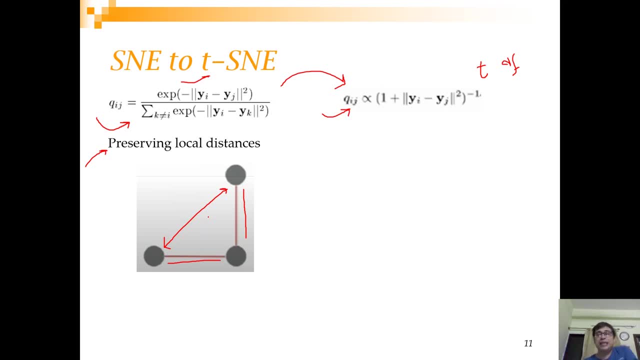 So now, if I want to represent it in a 1D plane so that this local distance is preserved, What can be a representation is something like this: OK, So you can see easily that both the local distances are preserved. However, what has happened to this maximum distance? 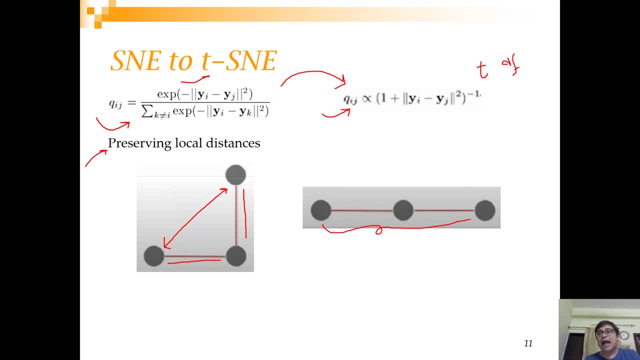 So this maximum distance has actually increased. OK, So when I am trying to preserve local distance, what I want is, you know, I want the large pairwise distances to go farther apart. So, from the high dimension representation, when we go to a low dimension representation, we want these to go farther apart. 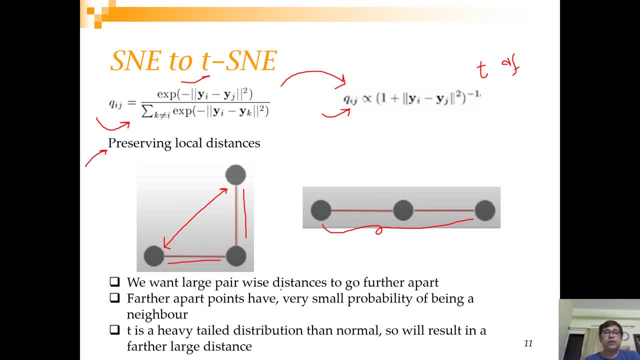 OK, And actually you know, if you follow the normal distribution, OK. So as you go towards the tail, OK, The probability becomes quite small, Right? So that means that as the distance from the reference point to the neighbor increases, the probability also goes down. 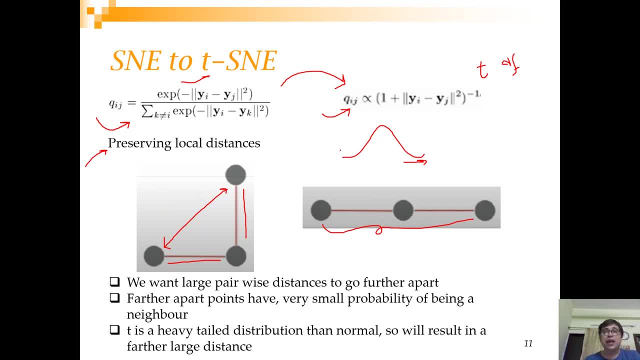 And in case of T distribution, if you remember that T has a farther strong tail, So T distribution looks something like this: OK, So to get a similar probability here. So what can be, you know, in normal distribution? OK, Getting a very, very small probability. 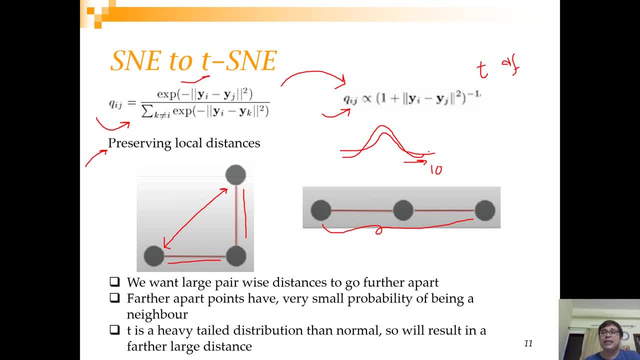 If you go, If you had to go to a distance of 10 in T distribution, you will have to go to a distance of 30. Right, So this will help us to actually, you know, put more weight to this large pairwise distances. 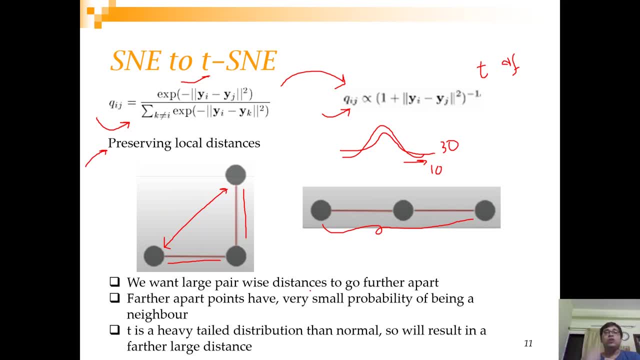 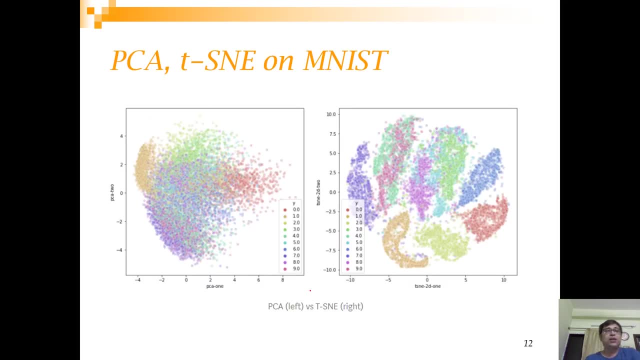 OK, So that actually motivated the authors to move from S&E to TISNI. Now let us look at a visualization. OK, With PCA and TISNI. So this is on the famous MNIST dataset. OK, So you know, these are the two first PCA dimensions and the classes are marked in same color. 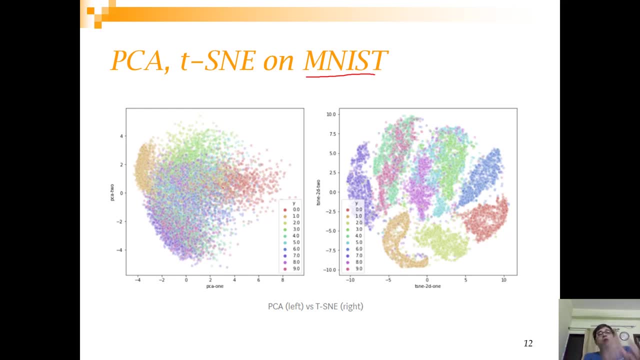 So you see that, and you remember that MNIST is about 10 digits, Right, So, from 0 to 10.. OK, From 0 to 9.. OK, And these are represented by different colors, All right. So, PCA, you see that they have gone all over places. 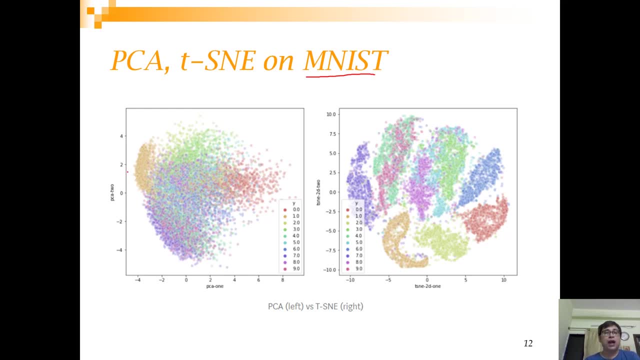 Only some of them maybe one could have identified clearly, Whereas TISNI Has beautifully separated them out, Right? So please remember both of them are unsupervised. Only the color information has been used to color code them, not for anything else.